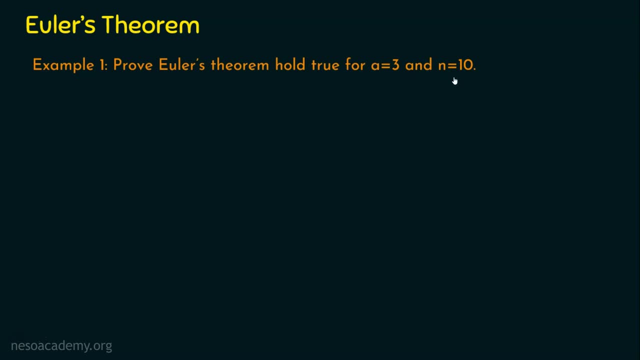 is 1.. Is 1 is the only number that can divide both 3 and 10?? Yes, 1 is the only biggest number that can divide both 3 and 10.. So obviously Euler's theorem will hold true for these values. Anyway, let's prove that. now We know the given data are: a is equal. 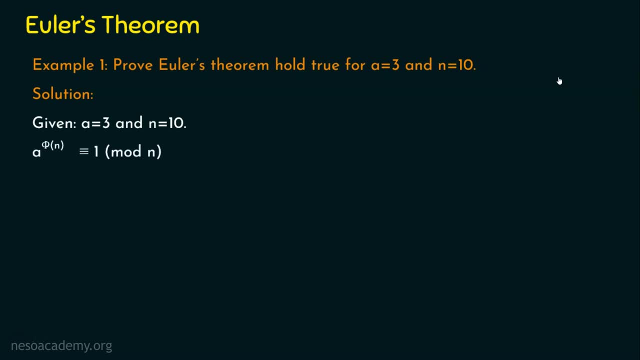 to 3 and n is equal to 10, and Euler's theorem states that a power phi of n is congruent to 1 mod n. Now what is n? 10.. So we will just substitute the values of a and n in the respective 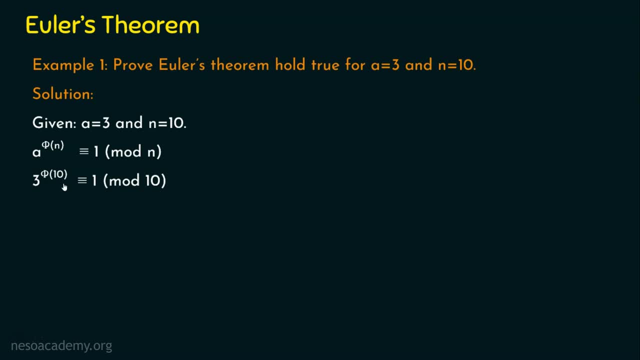 form of a and n. Now, if you note, here we are going to find phi of 10. We have already solved this in the previous lecture. Phi of 10 is equal to 4.. How did I get this? I hope you can recollect. 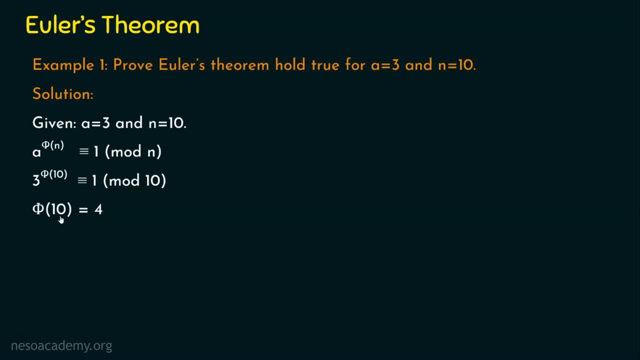 this. I have given some formulas to solve this. See, 10 can be a product of two different prime numbers: 2 and 5, right? So 10 can be written as 2 into 5.. So 2 and 5 are two different prime. 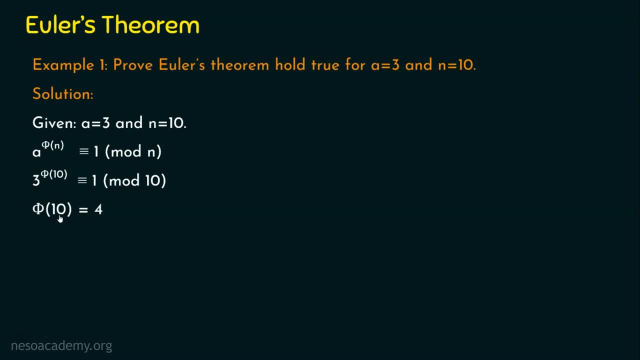 numbers. When you are going to compute phi of n, where n is a product of two different prime numbers, pq, the formula is: phi of n is equal to p minus 1.. Here 2 and 5 are the prime numbers, So obviously 2 minus 1 into 5 minus 1.. So 2 minus 1 is 1 and 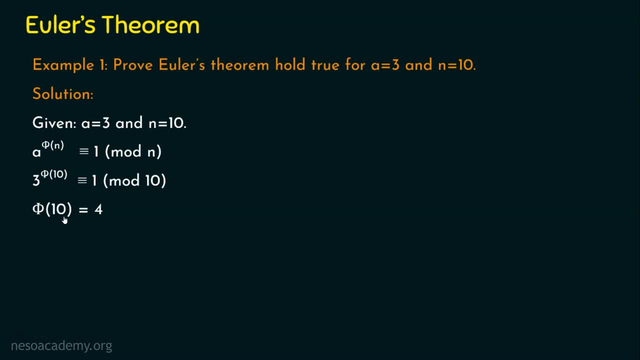 5 minus 1 is 4.. So 1 into 4 is 4.. If you are directly watching this lecture without knowing the basics of phi of n, I request you to watch my previous lectures titled Euler's Torsion Function. 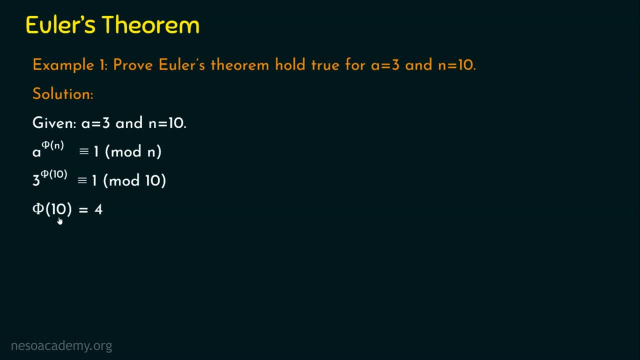 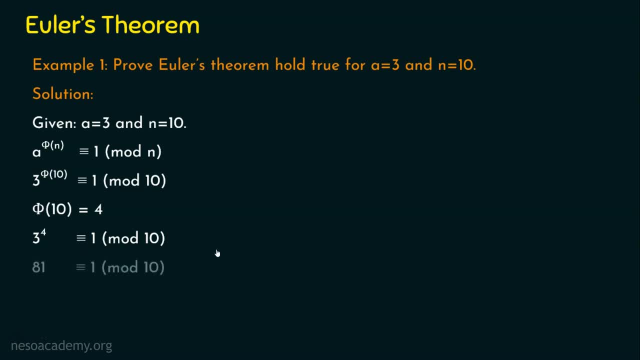 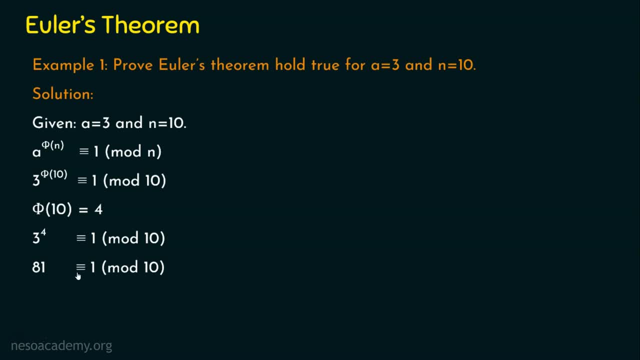 use the value of 3 power 4, which is 81. So 81 is congruent to 1 mod 10.. 81, when it is divided by 10, are we getting 1 as the remainder? Yes, Then 8 times 80 and obviously remainder is 1.. So 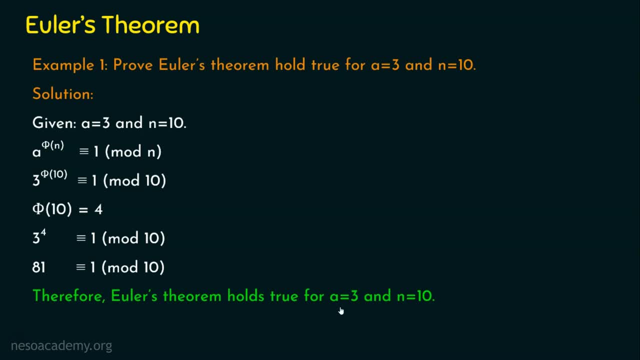 we can conclude that Euler's theorem holds true, for a is equal to 3 and n is equal to 10.. Let's see example number 2.. The question is: does Euler's theorem hold true, for a is equal to 2 and n is equal to 10? So we are required to check whether 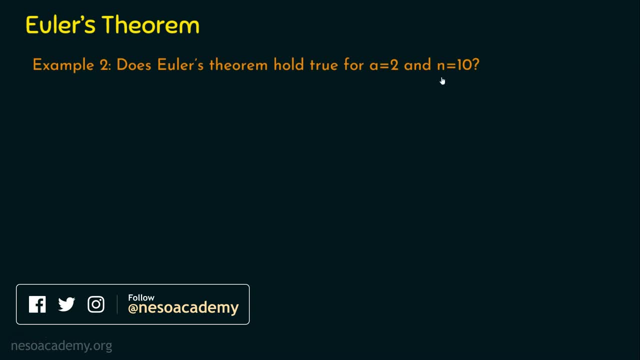 Euler's theorem hold true for these values. Let's analyze the initial conditions for every positive integer a. Of course a is a positive integer here, So no worries here Then. are 2 and 10 relatively prime to each other? No, When you perform GCD of 2 comma 10, we get 2 as the GCD. 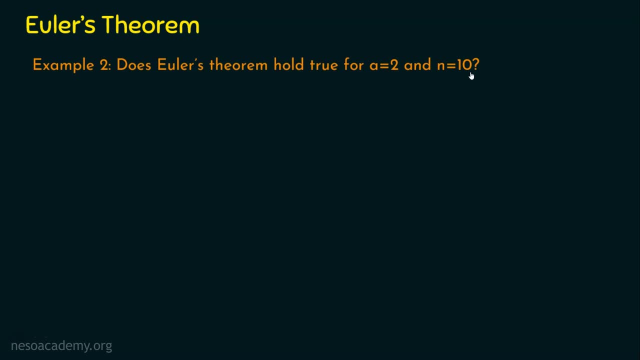 right, Because 2 is the biggest number, or the greatest number or the highest number that can divide both 2 and 10.. So obviously they are not relatively prime. From this we can easily conclude that Euler's theorem does not hold true, for a is equal to 2 and n is equal to 10, because 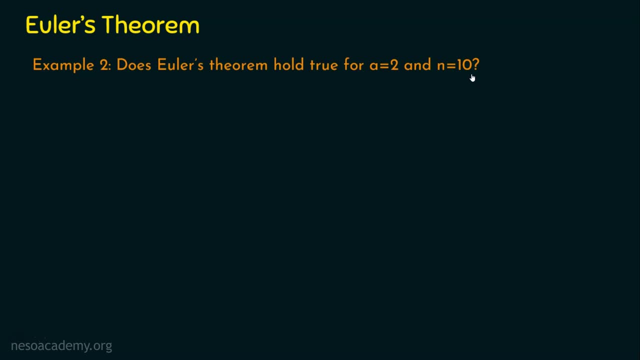 a and 10 are not relatively prime to each other. Anyway, let's prove that We know the given data are: a is equal to 2 and n is equal to 10. and we know what Euler's theorem states: It is a power. 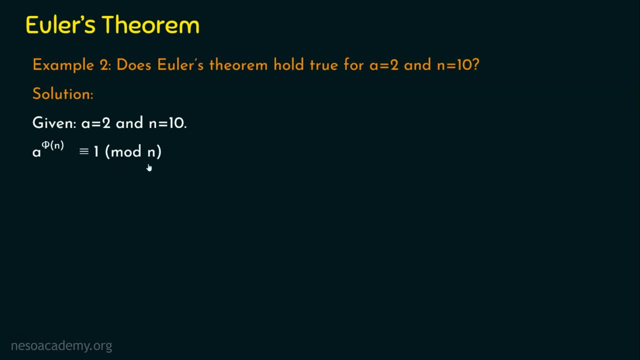 5 of n is congruent to 1 mod n. if a and n are relatively prime to each other, Let's substitute the values. We get 2 power 5 of 10 is congruent to 1 mod 10.. In the last example itself we solved 5. 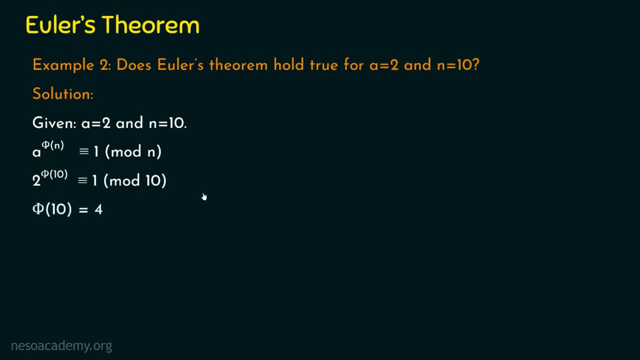 of 10, right, So we know the 5 of 10 value is 4.. We are going to use that value here directly. So 2 power 4 is congruent to 1 mod 10.. We will directly use this value: 2 power 4.. 2 power 4 is. 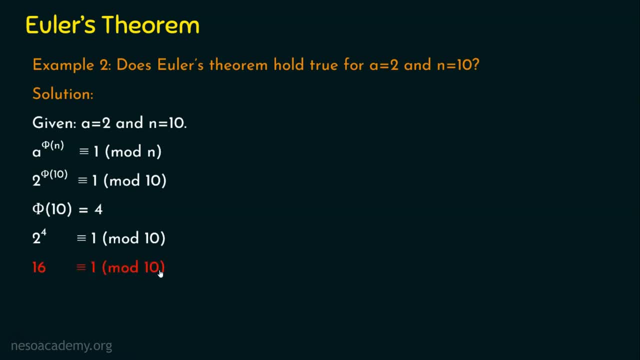 what 16.. So 16 is congruent to 1 mod 10.. You can see here this is an invalid congruence, because 16, when it is divided by 10, we get 6 as the remainder, not 1 as the remainder. So 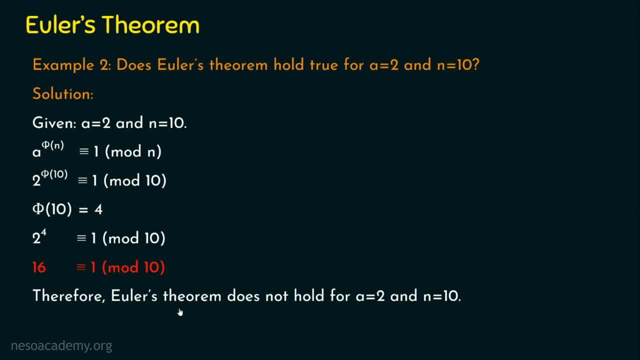 from this it's clear that Euler's theorem does not hold true, for a is equal to 2 and n is equal to 10.. The reason is a and n are not relatively prime to each other. Let's see the last example for the day, Example number 3.. Does Euler's theorem hold true? for a is equal to 10 and n is equal to. 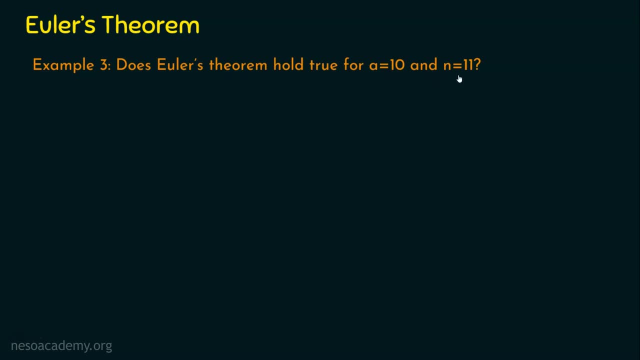 11?? Let's check whether a and n are relatively prime. Yes, a and n are relatively prime to each other, because the GCD of a comma, n, is 1.. So let's solve this. We know the given data are: a is equal to 10 and n is equal to 11.. We know. 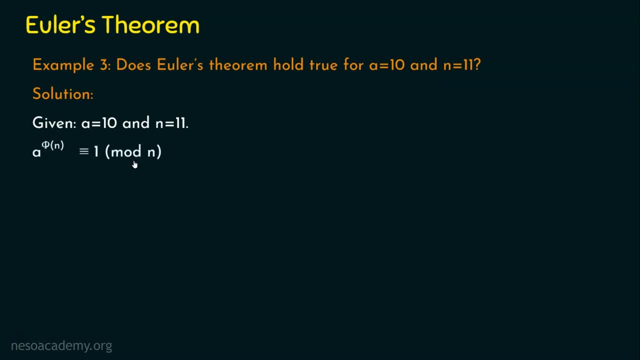 Euler's theorem states that a power 5 of n is congruent to 1 mod n when a and n are relatively prime to each other. We will substitute the values. We get 10 power 5 of 11 is congruent to 1 mod 11.. We are required to find 5 of 11, right? So 5 of 11 is equal to simply 10.. Why, If this? 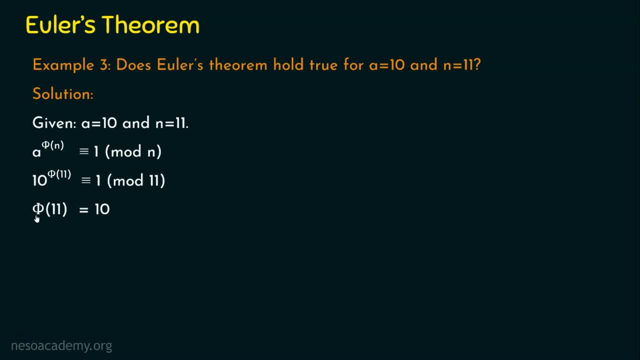 n is a prime number, then this is n minus 1, right, So 5 of n is equal to n minus 1. if n is a prime number, Here n is a prime number, So we get: 5 of 11 is equal to 10.. We will directly substitute the value 10. power 10 is congruent to 1 mod 11.. 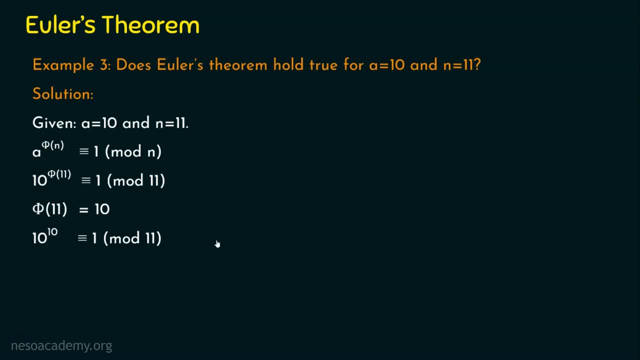 Are you going to solve this 10 power 10 using modular exponentiation? We can solve it. We will get the same result anyway. But can you see, here We can simplify this. This is 10 and this is 11.. We know this. 10 is minus 1 shortage from 11, isn't it? So we can simply write it as minus 1 power 10. 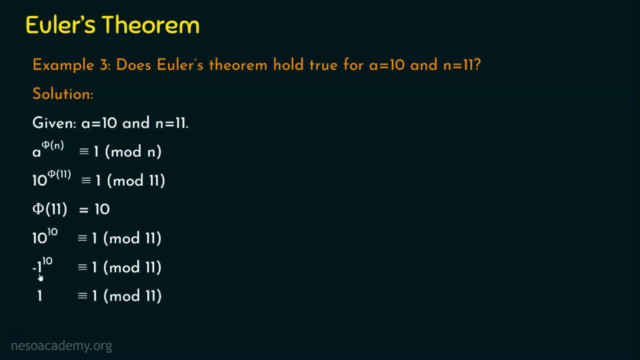 congruent to 1 mod 11. minus 1 to the power odd number, We get minus 1 itself. Since minus 1 power even number we have, we get 1.. Now let's check 1 divided by 11.. When you divide 1 by 11, we get. 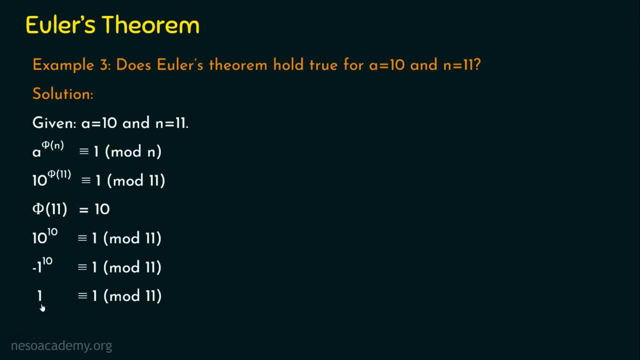 1 as the remainder, because 11 takes 0 times for 1.. So we get 1 as the remainder. So obviously Euler's theorem holds true, for a is equal to 10 and n is equal to 11.. Before we sign out: 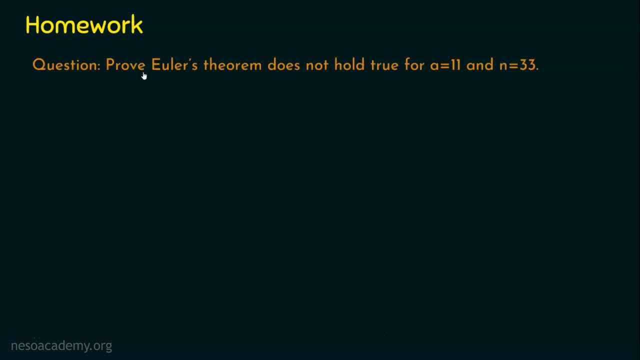 let's see the homework question. The question is: you are required to prove Euler's theorem does not hold true, for a is equal to 11 and n is equal to 33.. So before progressing with the solution, I request you to check whether a and n are relatively prime to each other. 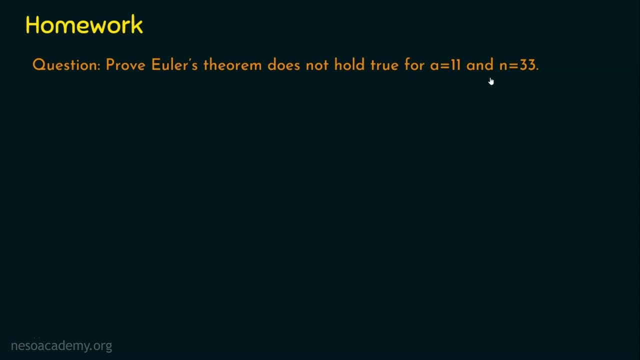 After knowing the answer by looking at the question itself. still, you prove this and post your answers in the comment section. And that's it, guys. I hope now you know what Euler's theorem states and the working of Euler's theorem with examples. I hope you guys enjoyed this presentation and thank you for watching.